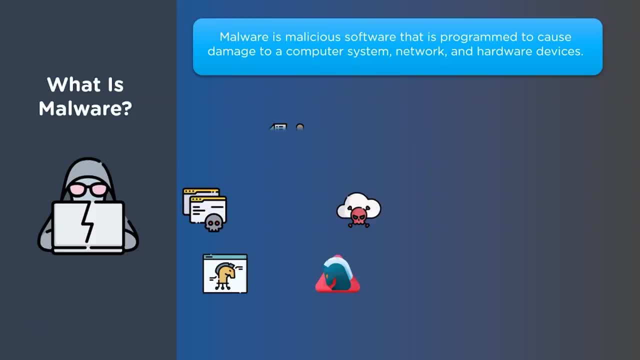 and hardware devices. Many malicious programs like trojans, viruses, bombs and bots, which cause damage to the system, are known as malware. Most of the malware programs are designed to steal information from the targeted user or to steal money from the target by stealing. 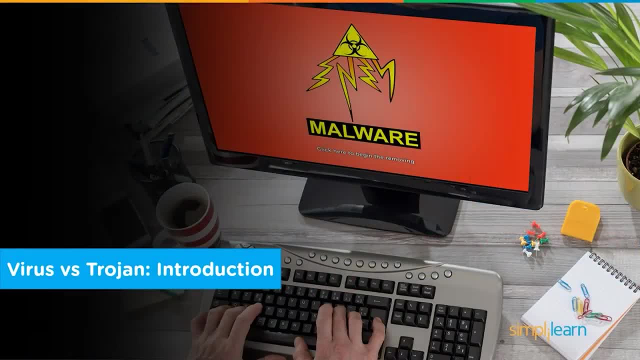 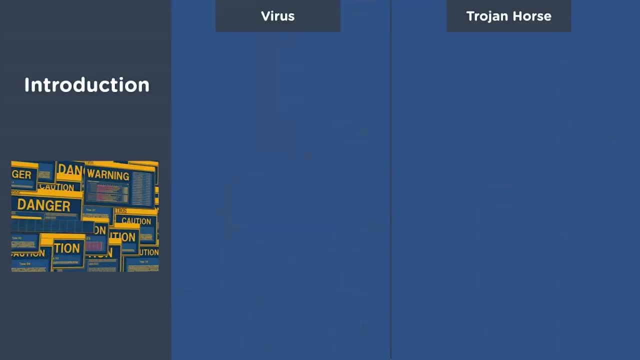 sensitive data. Let's take a look at the introduction of malware. Malware is a malicious software that is programmed to cause damage to a computer system, network and hardware devices. The malware program has two types of interactions: virus and trojan. Firstly, let's take a look at what exactly is a virus program. 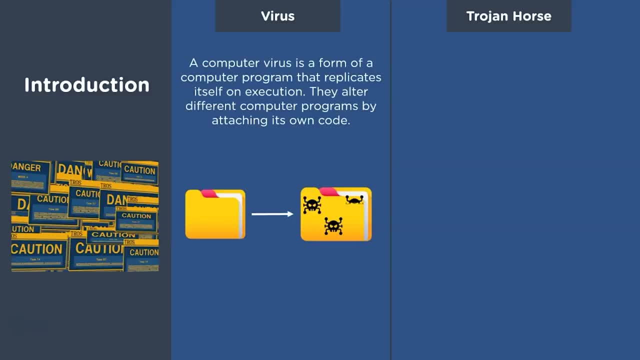 A computer virus is a type of malicious program that, on execution, replicates itself. They get attached to different files and programs, which are termed as host programs, by inserting their code. If the attachment succeeds, the targeted program is termed as infected with a computer virus. 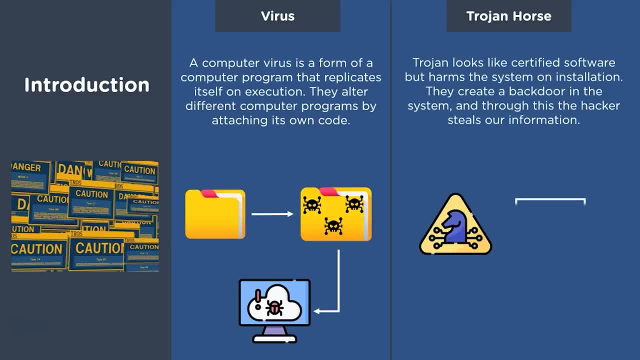 Now let's take a look at how the host programs work. take a look at the Trojan horse. Trojan horse program is a program that disguises itself as a legitimate program but harms the system on installation. they hide within the attachments and emails, then transfer from one system to 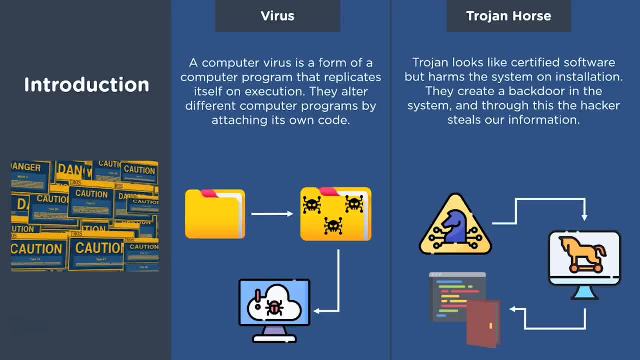 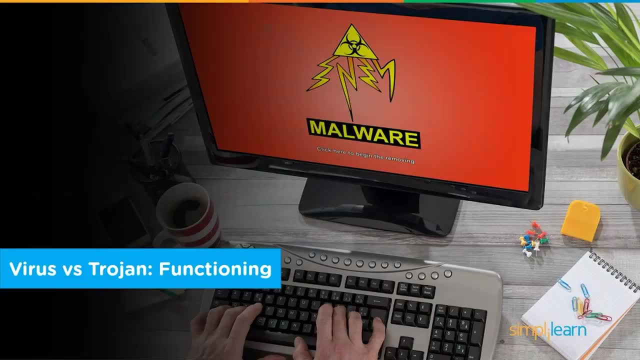 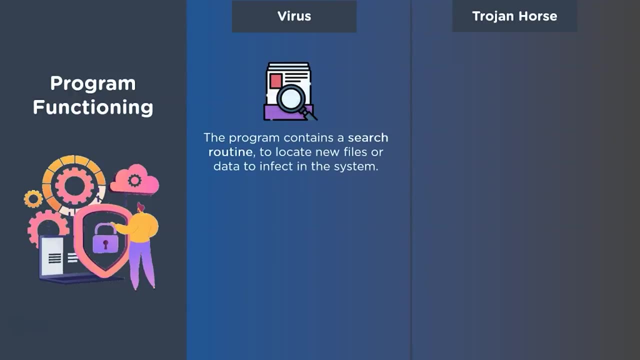 another. they create back doors into a system to allow the cyber criminal to steal our information. let's take a look how they function after getting installed into a system. firstly, we have virus programs. the computer virus must contain two parts to infect the system. first is a search routine which locates 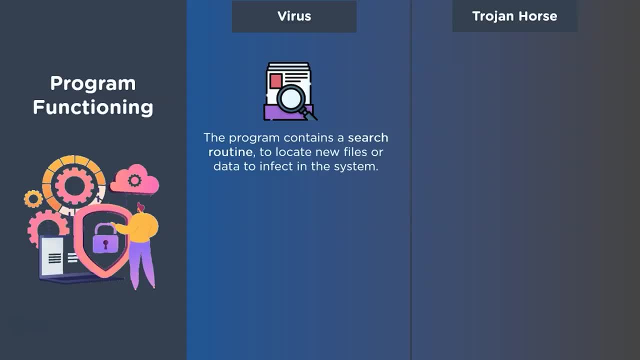 new files and data that is to be infected by the virus program, and the second part is known as the copy routine, which is necessary for the program to copy itself into the targeted file, which is located by the search routine. now let's take a look at the Trojan horse functioning. 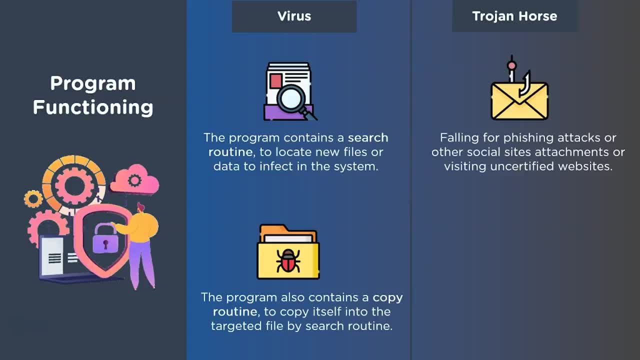 for Trojan horses. entry way into our system is through emails that may look legitimate but may have unknown attachments, and when such files are downloaded into the device, the Trojan program gets installed and infects the system. they also infect the system on the execution of infected application or 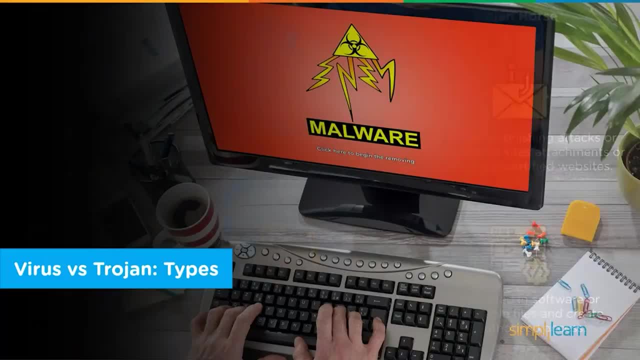 the executable file and attacks the system. now that we understand what virus and Trojans are, let's understand different types of virus and Trojans. now that we understand what virus and Trojans are, let's understand different types of virus and Trojans. 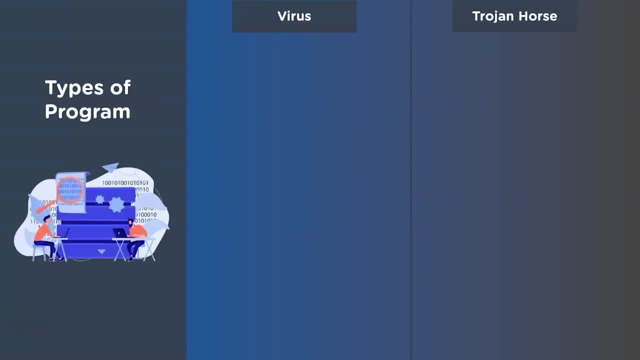 let's take a look at different types of viruses. the first one is known as the boot sector virus. this type of virus damages the booting section of the system by infecting the master board record, which is also known as MBR. this damages the boot sector section by targeting the hard disk of the system. then we have the 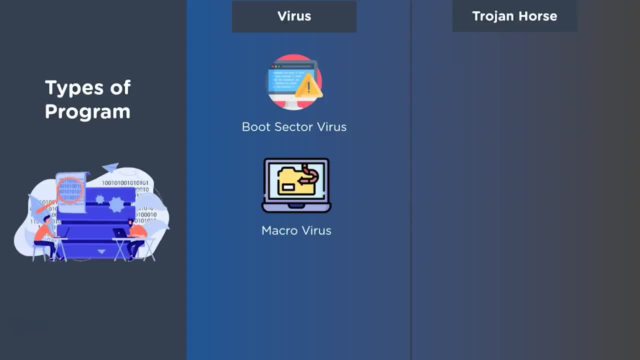 macro virus. macro virus is a type of virus that gets embedded into the document related data and is executed by the system. and the system is then executed by the system. and the system is then executed when the file is open. executed when the file is open. they also are designed to replicate. 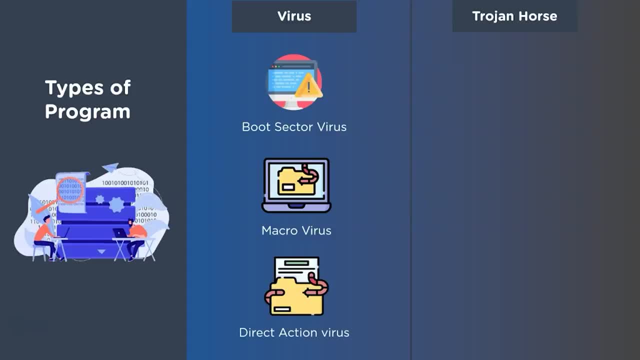 they also are designed to replicate themselves and infect the system on a larger scale. and lastly, we have the direct action virus. this type of virus gets attached to executable files which, on execution, activates the virus program and infects the system. once the infection of the file is completed, they exit the system, which is also the reason it is known as. 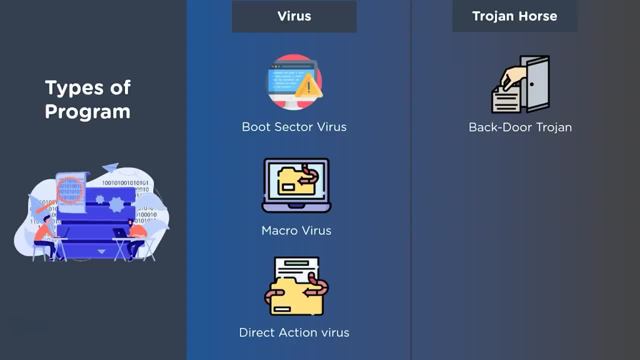 Let's take a look at different types of Trojans. The first type of Trojan is the Backdoor Trojan. They are designed to create a backdoor in the system on execution of an infected program. They provide remote access of our system to the hacker. 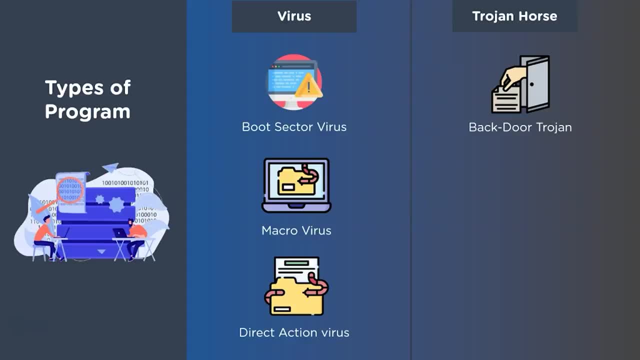 This way, the cyber criminal can steal our system data and may use it for illegal activities. Next, we have Crick-Sauced Trojan. They enter the system by clicking the random pop-ups which we come across on the internet. They attempt the user to give their personal details for different transactions or schemes. 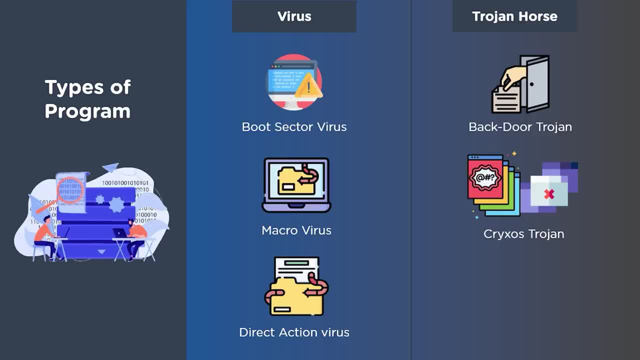 which may provide remote access of a system to the cyber criminal, And the last Trojan type is Ransom Trojan. This type of Trojan program, after entering the system, blocks the user from accessing its own system and also affects the system function. The cyber criminal demands a ransom from the targeted user for the removal of the Trojan program from the device. 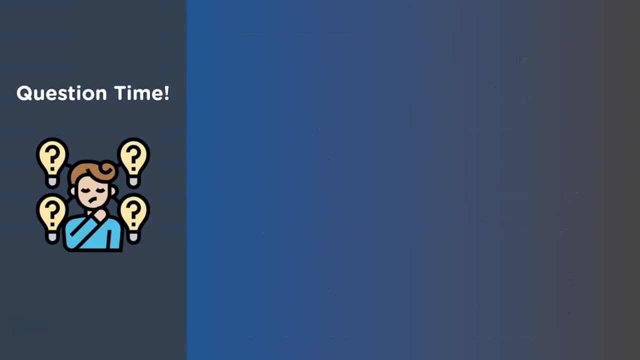 Now that we understand some details regarding Viruses and Trojans, Let's solve a question. The question is: Jake was denied access to his system and he wasn't able to control the data and information in his system. Now the actual question is: What could be the reason behind systems problem? 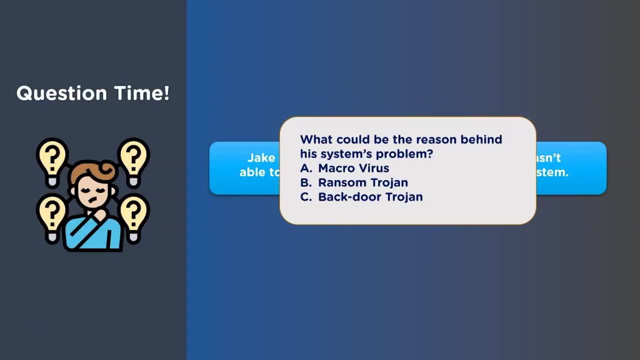 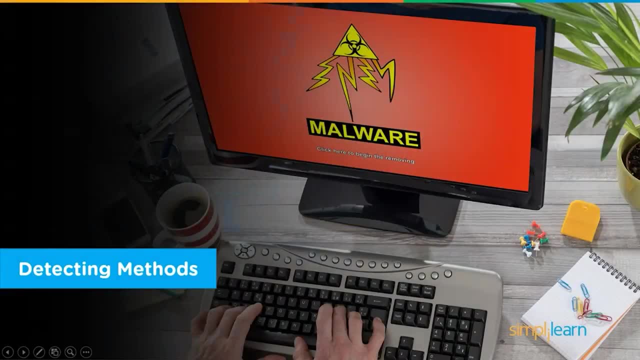 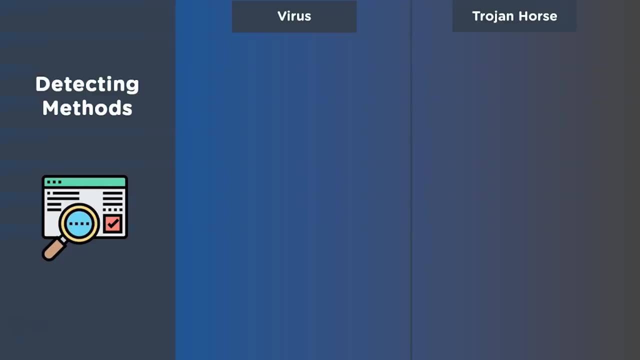 Option A: Macro Virus. Option B: Ransom Trojan. Option C: Bagdor Trojan. Give your answers in the comment section. Now let's understand how to detect the activity of viruses and Trojan in a system. To detect virus or Trojan activity in a system, we can refer to the following points. 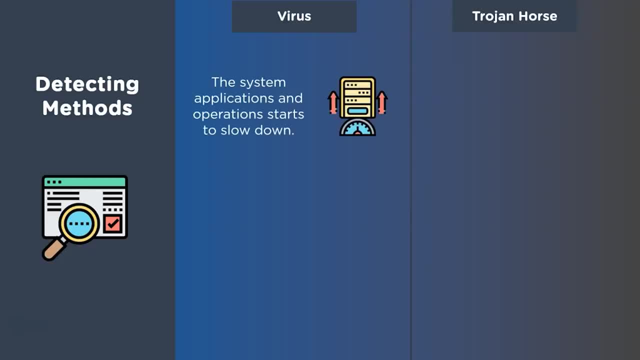 For viruses, we have slowing down of the system and frequent application freeze shows that the infection of the virus is present in the system. Then we have the viruses can also steal sensitive data, including passwords, account details, which may lead to unexpected logout from the accounts or corruption of the sensitive data. 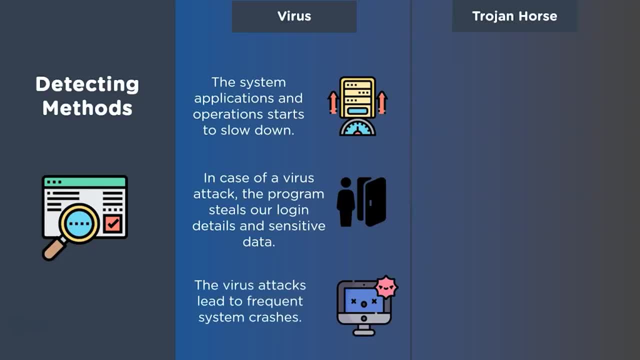 And lastly, we have frequent system crashes due to virus infection which damages the operating system For Trojan. we have frequent system crashes and system also faces slow reaction time. Then we have there are more random interactions, There are pop-ups from the system which may indicate Trojan activity. 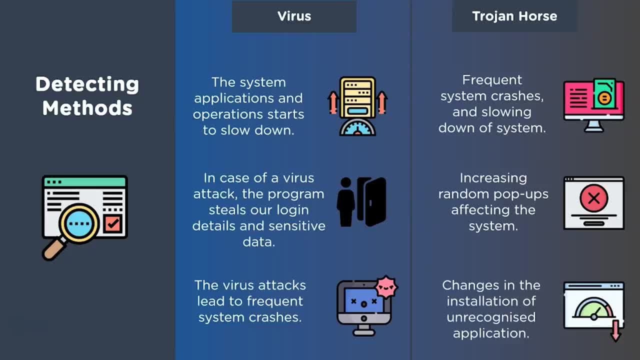 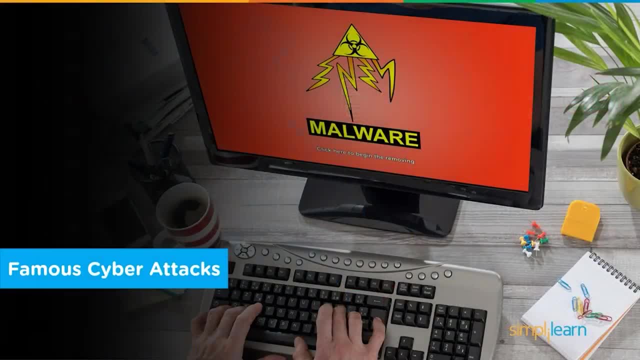 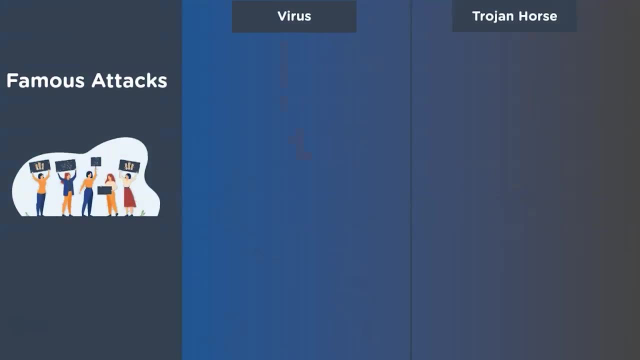 And lastly, we have modification in the system application and change of the desktop appearance can be also due to the infection of a Trojan program. Next, let's take a look at a famous cyber attack for virus and a Trojan horse For virus. we have the MyDoom virus, which was identified in the year 2004, which affected over 50 million systems. 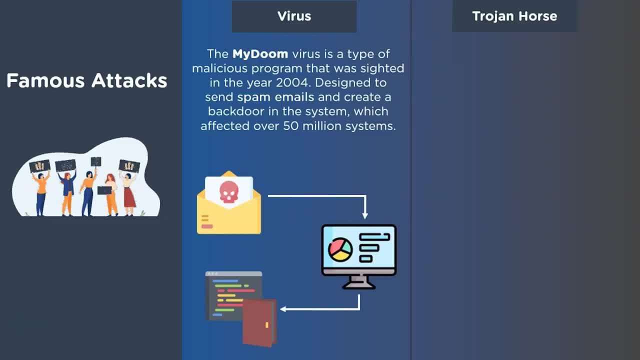 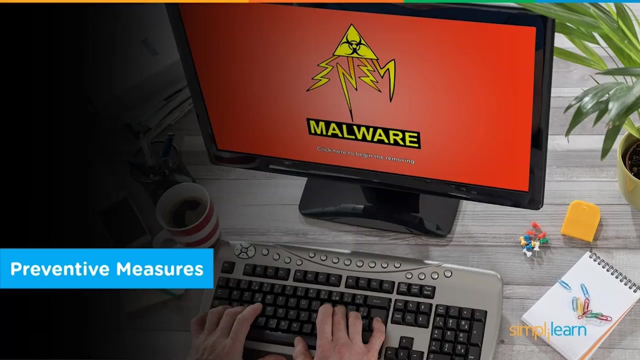 By creating a network of sending spam emails, which was to gain backdoor access into our systems. Next, for the Trojan horse, we have the Emotat Trojan program, which is specifically designed for financial theft and for stealing bank-related information. Next, we have a few points for how to prevent virus entry or Trojan attack for our system. 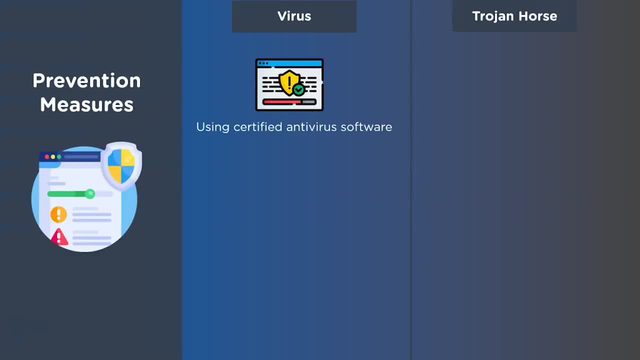 The most basic way of virus protection is to use a system called the Emotat Trojan program. The most basic way of virus protection is to use a system called the Emotat Trojan program. The most basic way of virus protection is to use a system called the Emotat Trojan program. 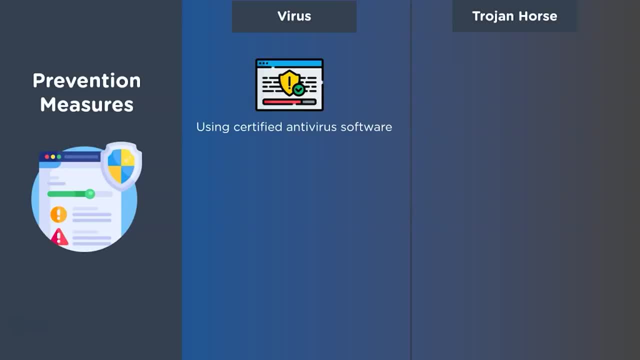 The norm is to use an antivirus and do regular virus scans. This will prevent virus entry into our systems, and also, having more than one antivirus then avoid visiting un-certified websites and this will also prevent virus entry into our system. Then we have using regular driver updates and system updates to prevent virus entry.